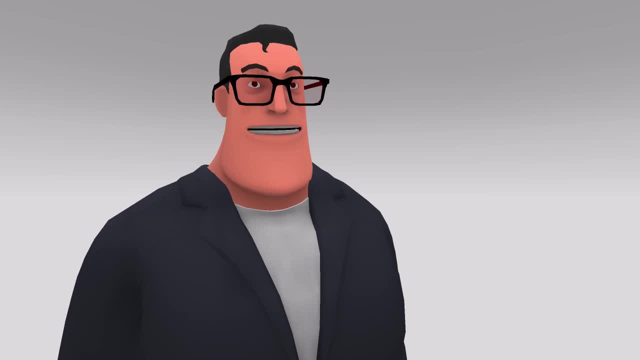 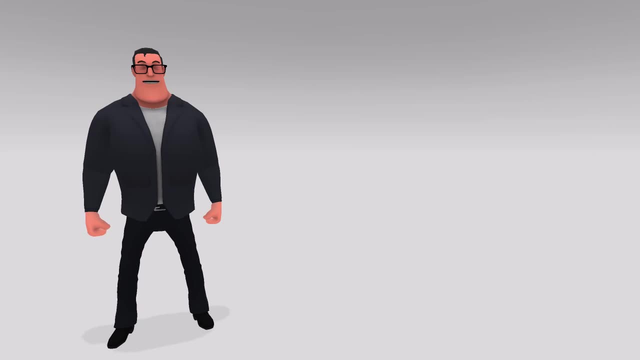 in very simple terms so that you can take the best decision about this dilemma. but before that, please read this disclaimer. There are many myths in the market about low strength power eyeglasses, For example. wearing low strength power eyeglasses will worsen your 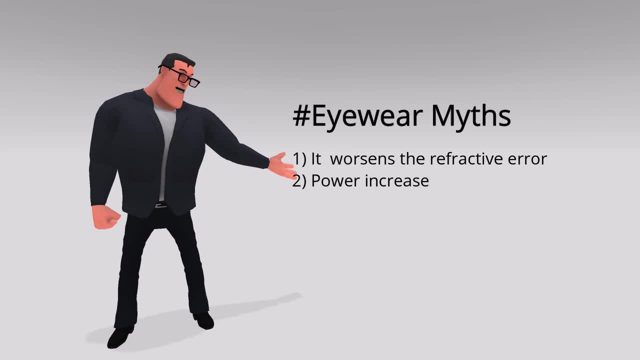 refractive error. Some people also say that not wearing the eyeglasses could become the reason of high refractive error in future. Even if you wear the low diopter eyeglasses, you will not be able to work without that and become dependent on eyeglasses. Well, 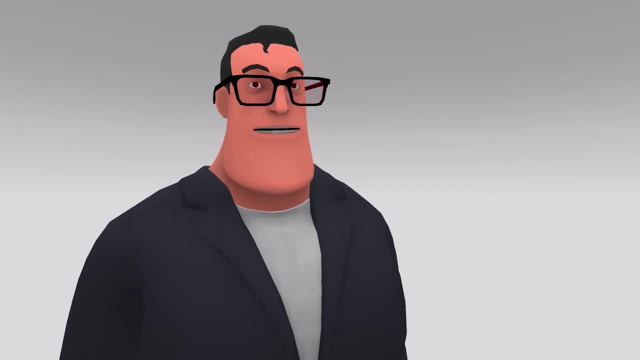 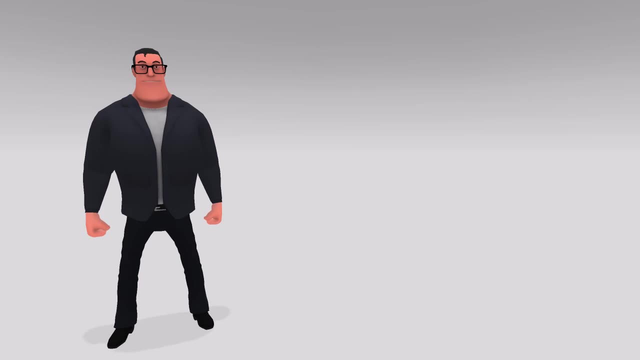 none of the points above are true. Let's understand what it means if a doctor has prescribed you a minus 0.25 or minus 0.50 eyeglasses. It simply means that the subject can read the 8th line of Snellen chart from a distance. 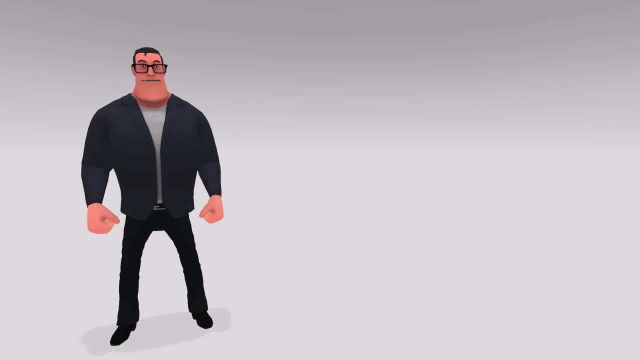 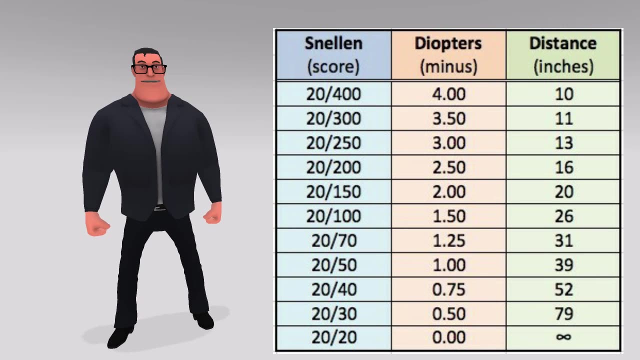 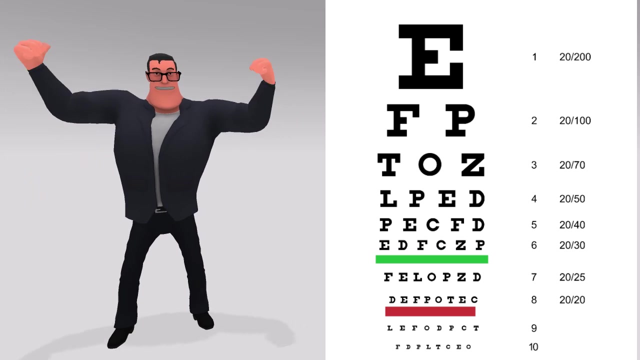 of 20 feet. If your prescription reads minus 0.25 diopter's spherical power, then your Snellen score is 20.25.. This score means that while eyesight examination you could read only till 7th row of Snellen chart from the distance of 20 feet. However, a person with normal vision, or perhaps a fighter pilot, can read the 8th line of Snellen chart from a distance of 20 feet. If your prescription reads minus 0.25 diopter's spherical power, then your Snellen score is 20.25.. This score means that while eyesight examination you could read only till. 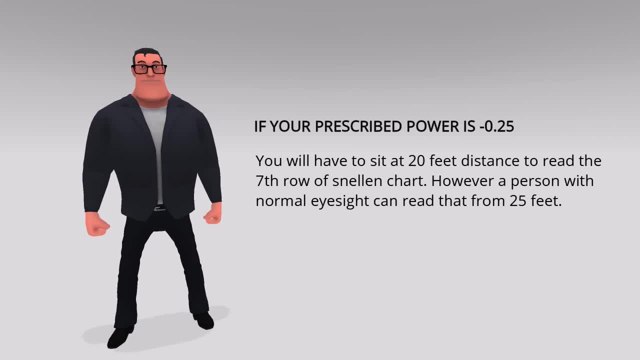 7th row of Snellen chart from the distance of 20 feet. However, a person with normal vision, or perhaps a fighter pilot, can read that row from 25 feet, which is 5 feet away from your position. So what does this prove? It proves that technically, there is a little. 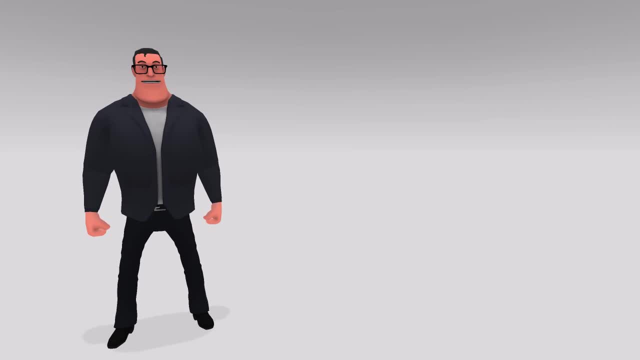 refractive error in your eyes. But hold on in normal daily life, how many of us are required to read such small alphabets? and that, too, from a distance of 20 feet? And you know what? There are some factors which can also influence the final result and give a false positive. 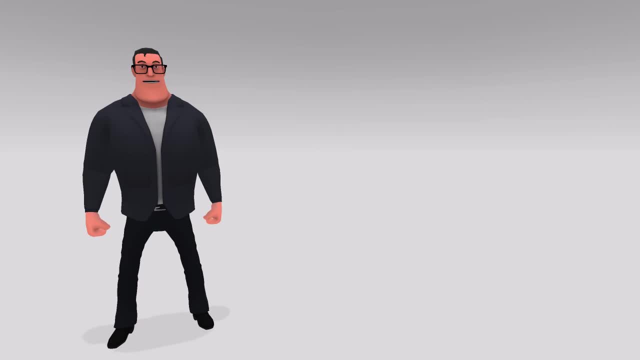 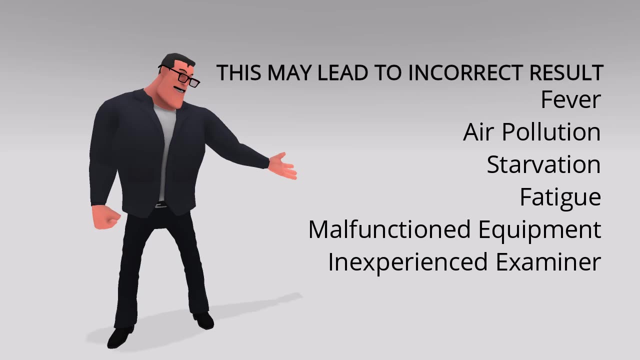 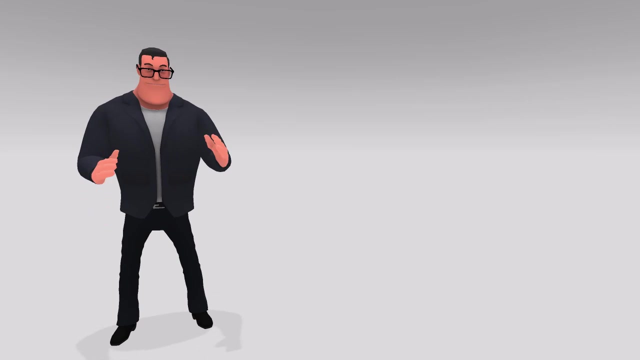 say, between minus 0.25 and minus 0.50 spherical diopters. For example, fever, air pollution, starvation, fatigue, malfunction equipment, inexperienced examiner, etc. There is a great possibility that you will encounter with at least one of those factors that could give.